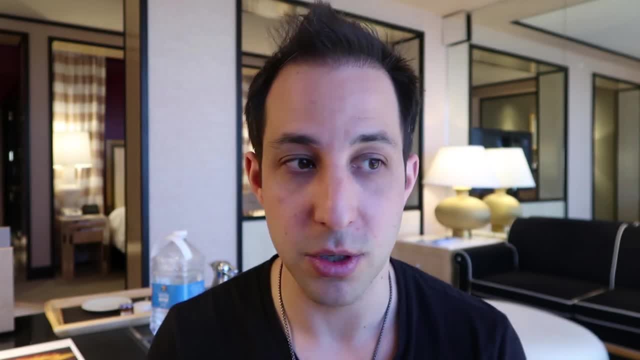 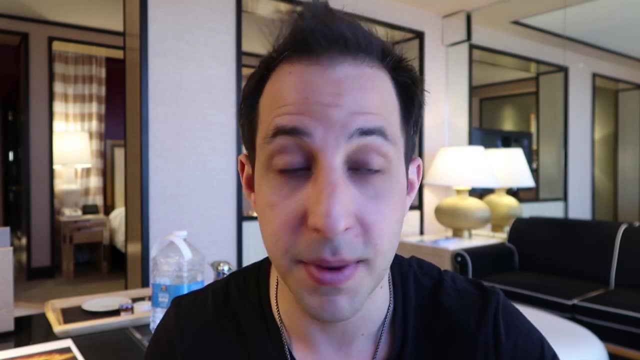 comments about the last video that these people in the street performers are not trying to do that. Their goal is to make as much money as possible on every single performance because they don't have repeat customers, right? If I told you, these street performers I saw sucked, don't go see them. 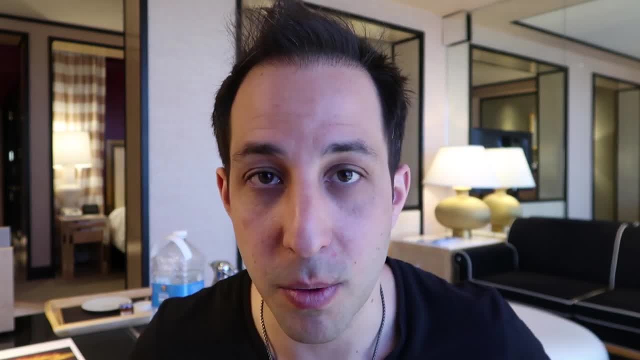 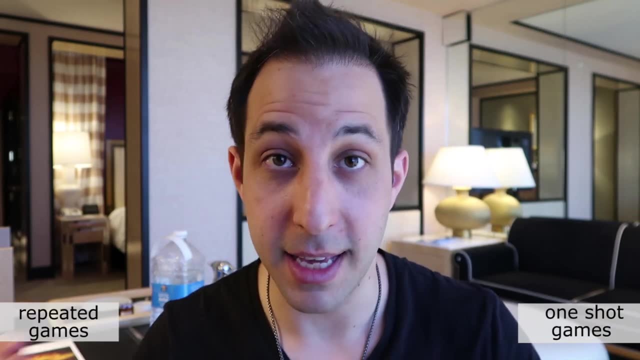 or don't pay them money. in New York City, what are you going to do? There's a million street performers. You're never going to find the same ones, And it led me to reflect on this idea that there's a difference between one-shot games and repeated games. 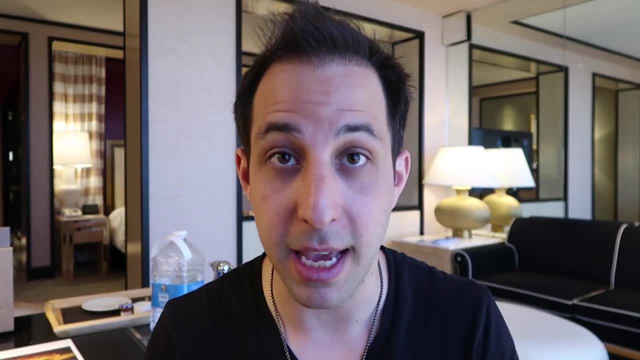 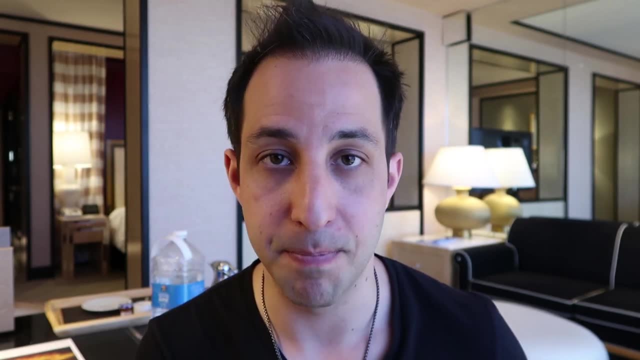 Poker teaches us this, and it's a lesson. I learned a lot in poker about how to play poker in different scenarios, And there are times you find yourself in a poker hand where you're playing a one-shot game. What do I mean by that? A one-shot game is a situation that exists in a vacuum. It's only 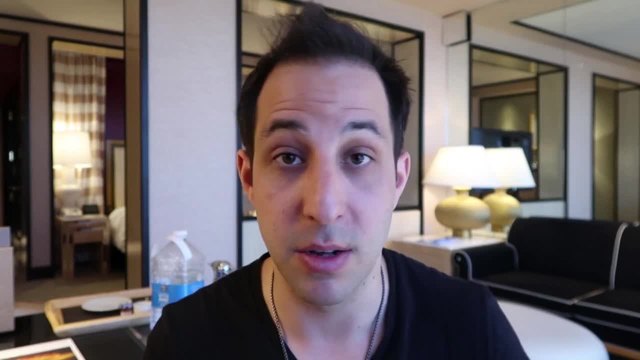 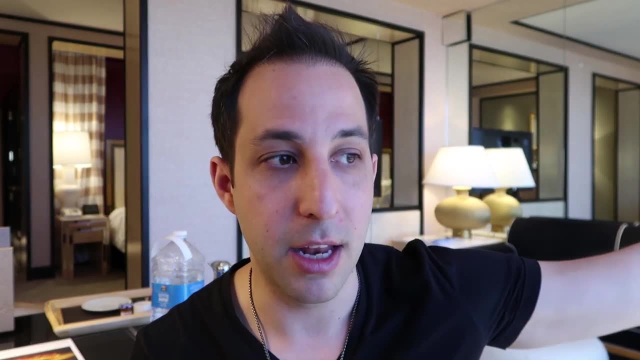 going to happen once. You're not going to run that situation or simulation thousands of times. An example: you're playing in a tournament, you're at the final table. you're playing against a guy from Switzerland and you've never played a hand with him before and you're at the final table. 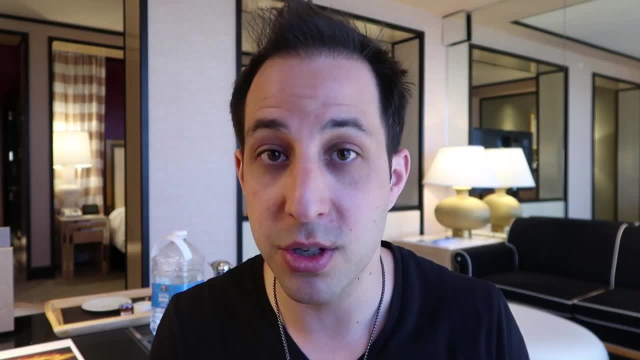 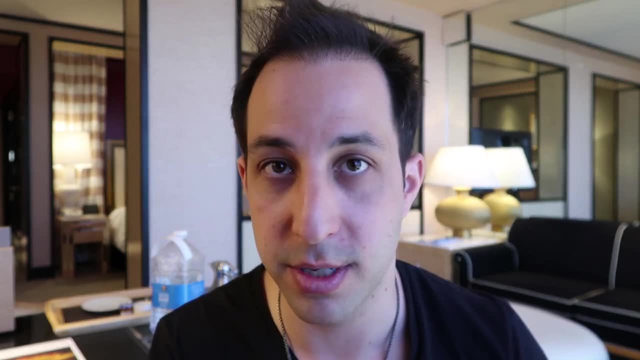 you're not going to play hands with him again in the future, You would be well served to just do everything you can to get the maximum edge and exploit him the most. if you think you can get away with some crazy play, that if he catches you you won't be able to make a second time, but you only. 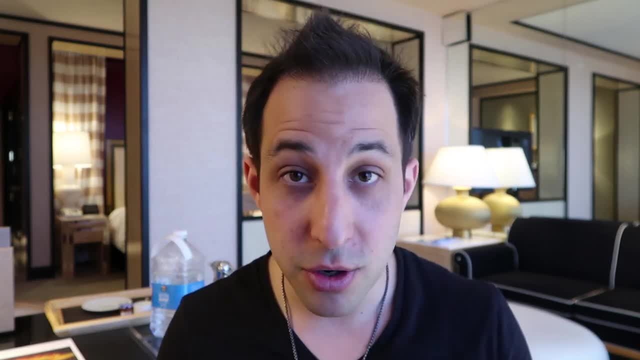 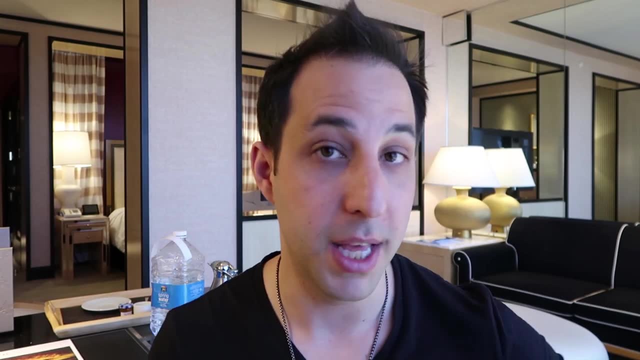 have the opportunity to make it once. This is a one-shot game. There are other circumstances in poker where you're playing repeated games. For example, you go to your local casino that you play at four times a week. you play against the same five or six regulars. You can't just do these. 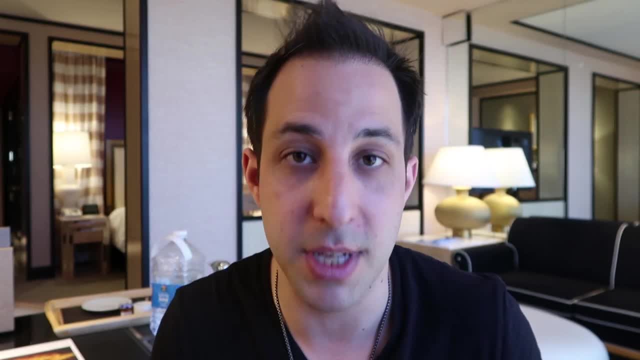 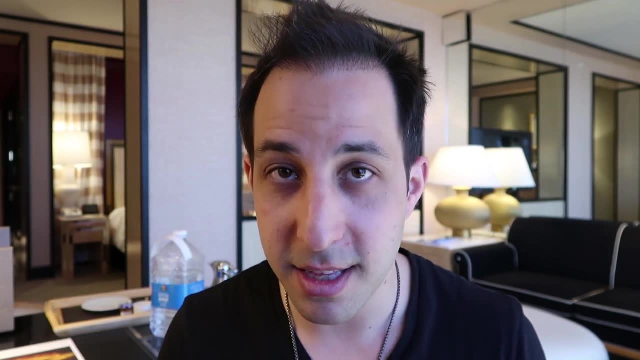 one-off plays and hope to get away with it, because if you do them multiple times and you keep trying to go back to the well, good observant players will notice this and they'll make adjustments. Most things in life are repeated games. You play sports, you watch tennis. you can't. 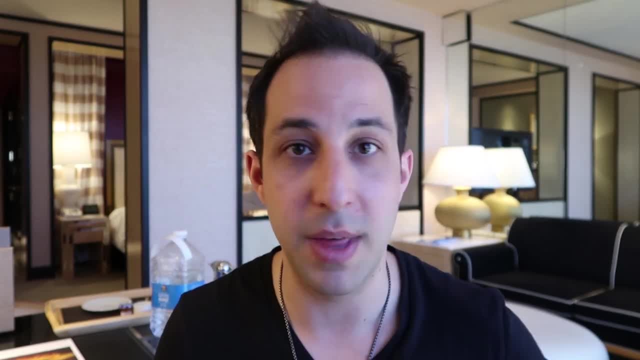 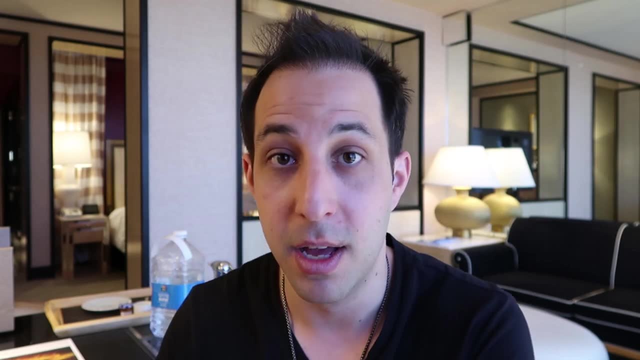 just hit a ball and then like serve and volley and do that every single time because you have to mix it up. Your opponents are going to catch what you're doing. You can't just serve the ball in the same place every time, because your opponent's going to know and he's going to move and adjust. 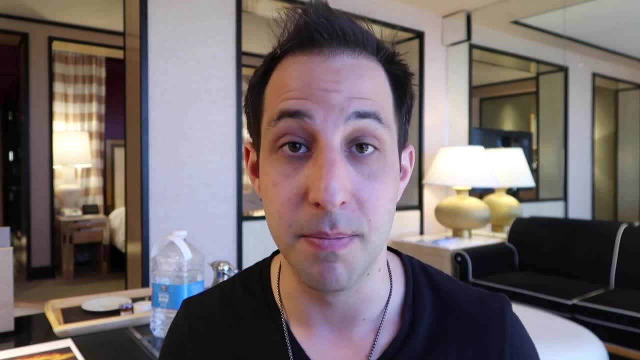 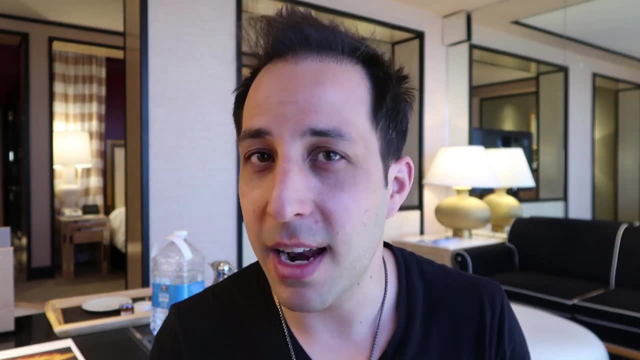 and then your serve will not be effective. So what you have to do is adopt a mixed strategy, But, most important, this is what game theory teaches us. But how does this really apply to life? Well, life is not a one-shot game, And aside, 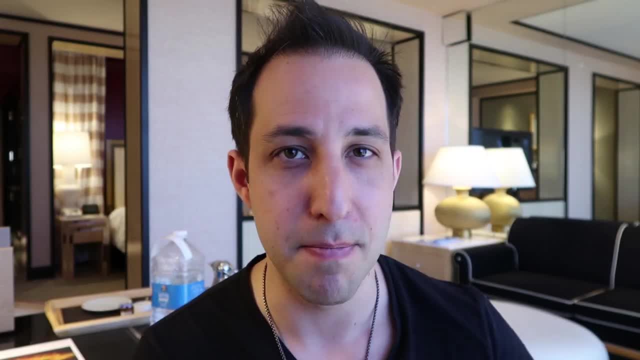 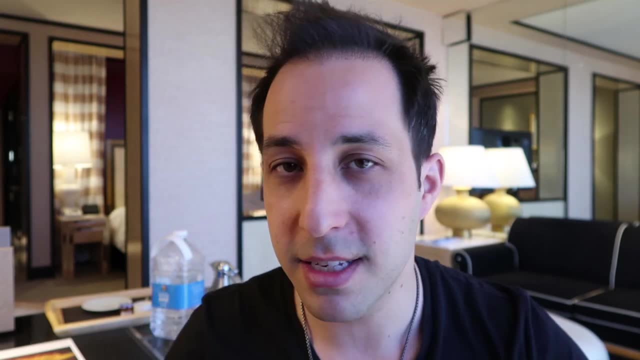 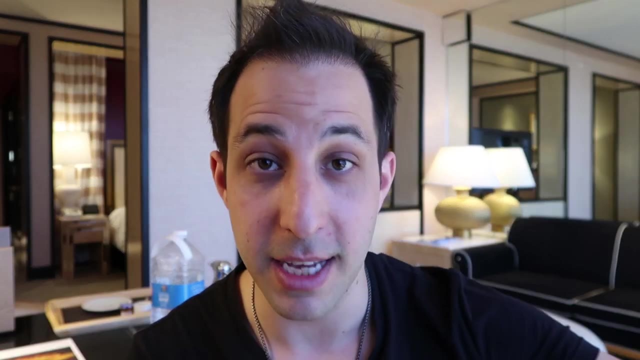 from these street performers, or rare examples where your objective is to maximize this specific situation without having any consideration for the long term. most things in life are repeated games. In other words, you're playing them for the long term and your long-term strategy is more. 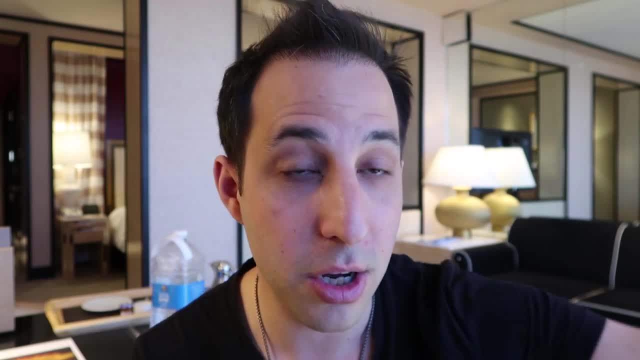 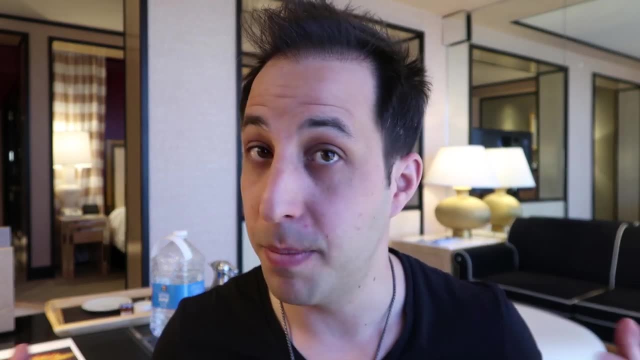 important than your short-term strategy. So what you have to do is adopt a mixed strategy And you're going to have a short-term opportunity. Your long-term opportunity to gain is more important than the short-term sale, For example, in branding or business. it means that building 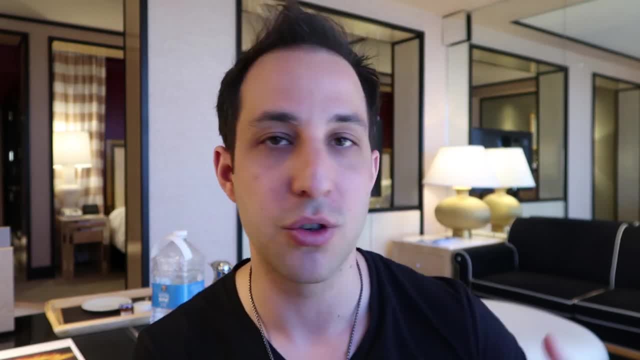 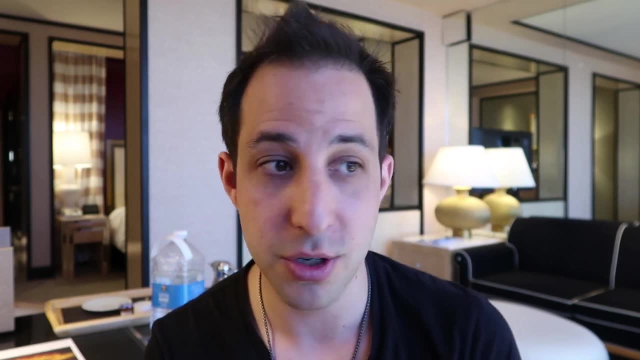 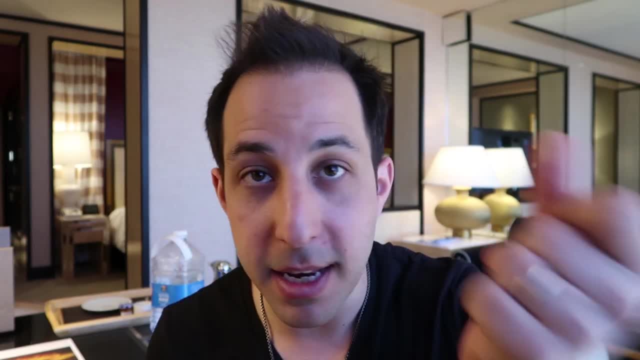 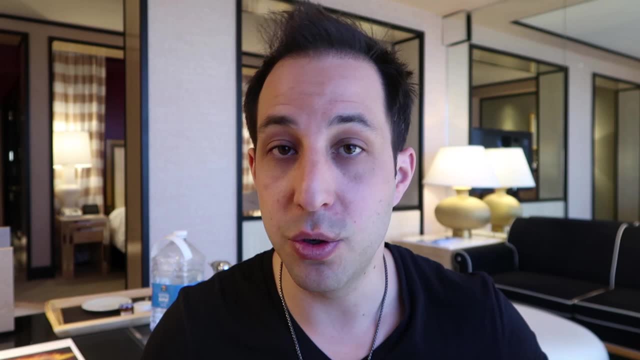 make a mistake, And you're going to have to make a mistake, And you're going to have to make a mistake. Their ads are directly focused on immediately going for the sale. They're asking for something. They're saying, hey, this is our product, We're the best, We're number one, Our shoes are made in. 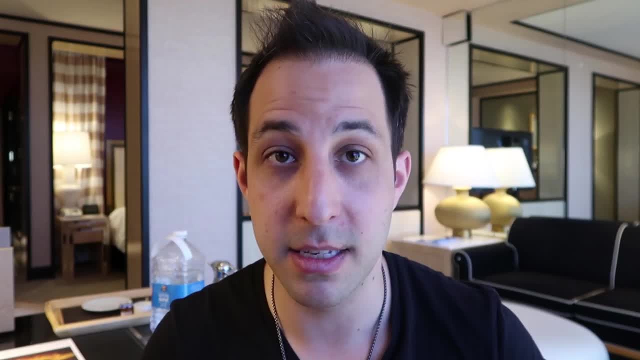 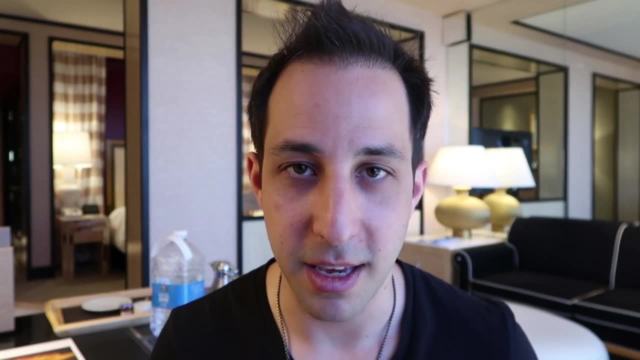 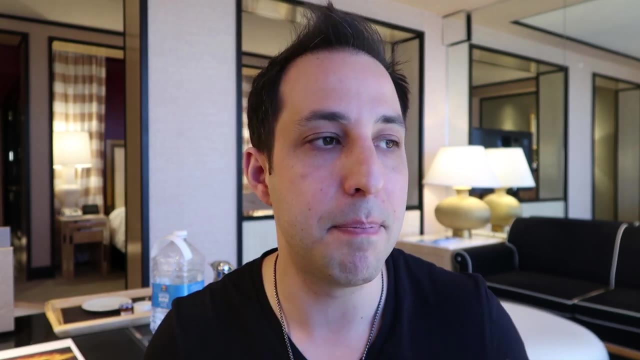 this way, from this fabric. They're cool. People say they're the best. Buy our shoes. It's a short-term game. They're going for the one-shot play. But what do great companies do Think about Nike? Their slogan is: just do it. They're selling you their vision about the world And you're not. 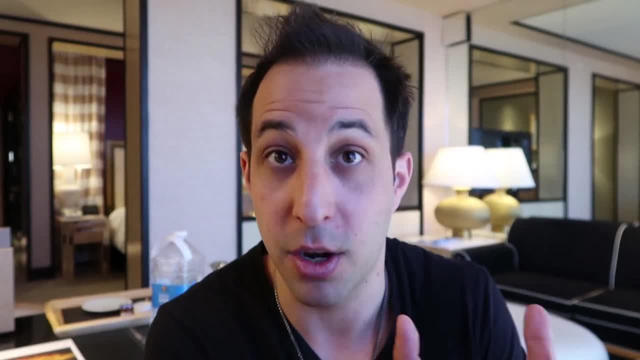 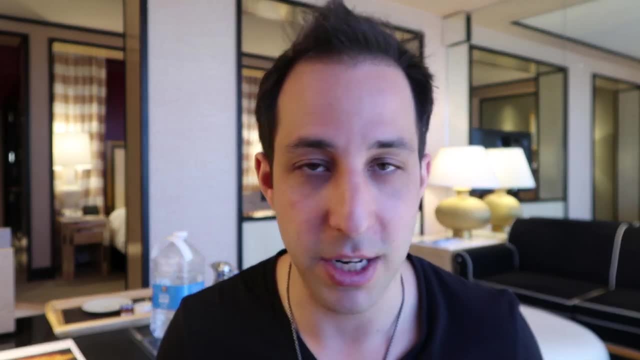 buying the fact that their shoes are stitched well. Of course they make a great product. If they made terrible shoes, nobody would buy them. They make great shoes, But every company would argue that they make great shoes And I'm sure a lot of companies can make great products. They. 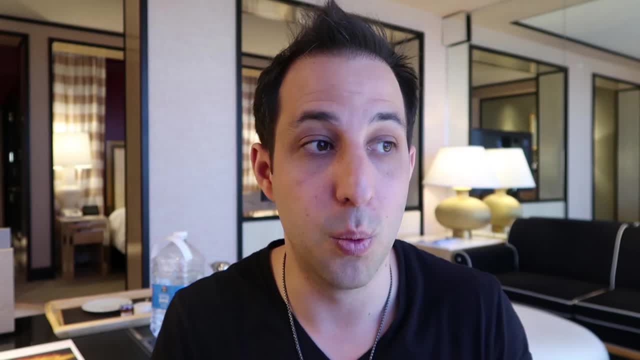 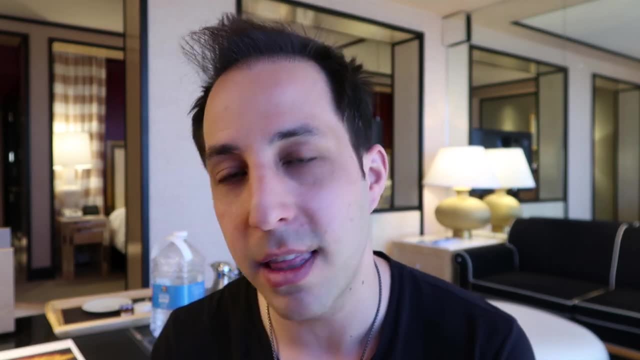 can make great t-shirts, But how does one distinguish themselves from another in a world where there's a sea of competition? They don't sell you what you're buying. They sell you why you're buying it: Because they're playing the long-term repeated game. Nike's latest commercial. 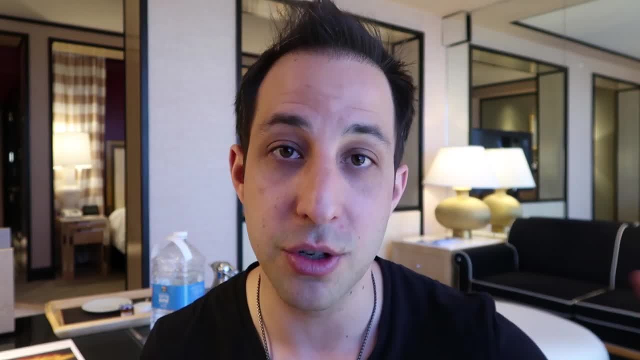 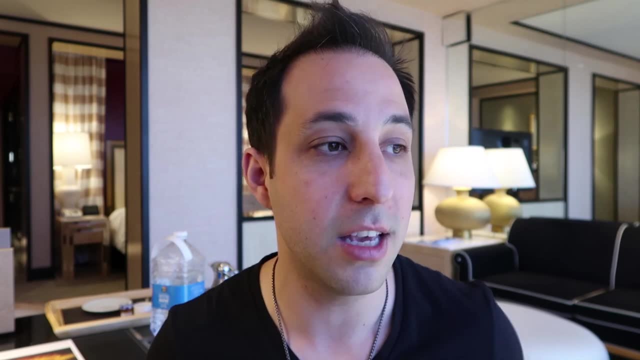 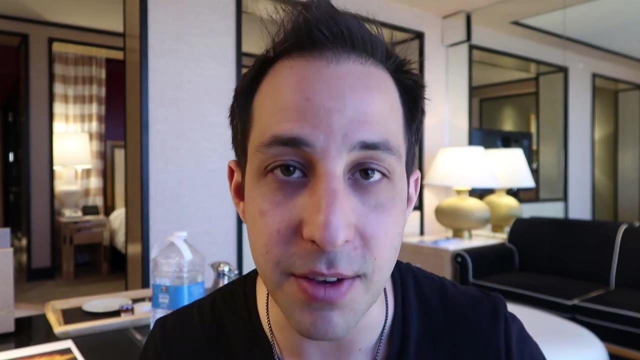 is write the future. Their campaign is: don't change your dream, change the world, Because they're selling you a vision. They're selling you a value system. They're selling you the fact that when you buy their product and you wear their shoes, you're expressing your belief of the world.